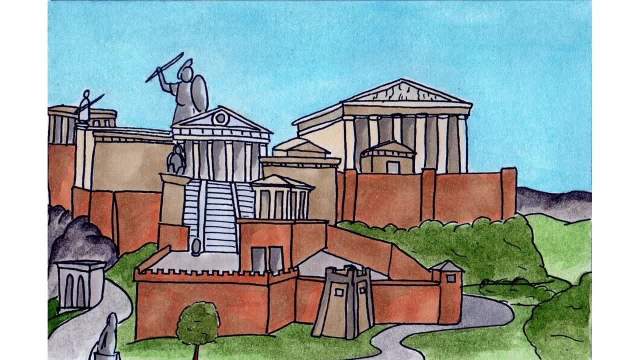 the Acropolis is its name, with its orderly collection of temples and shrines, their polished white marble and brightly coloured paint catching the eye. There in the middle is the Parthenon, the greatest building of the age, with its towering columns that could be seen for miles around. Ah, Athens, Even Delphi, who had 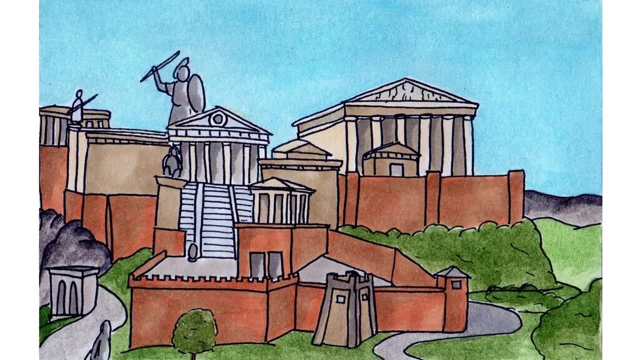 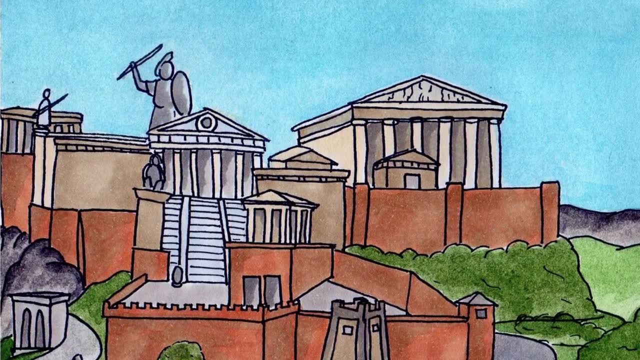 lived here all her life. in fact, she had been born in the house she had just left, knew in her bones that it was the most wonderful city in the whole world. As we turn our interest back to the dark-haired girl skipping down the road barefoot, we can see the little look of pride she carries with her. 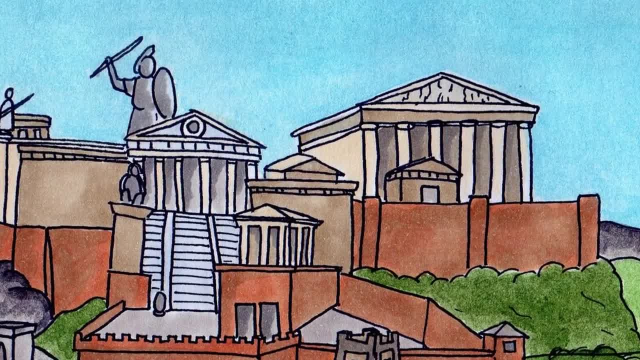 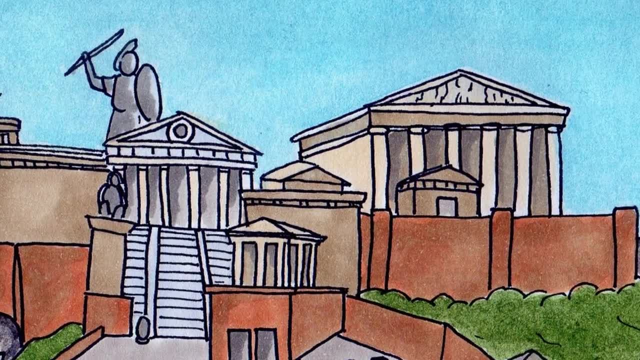 like a lucky charm. She loved her home and thought that it was her home and that she thought about it often. How terrible it must be to come from some other, less-cultured place. She leapt over a pile of horse-poo in the road and headed past the gymnasium, where the men would 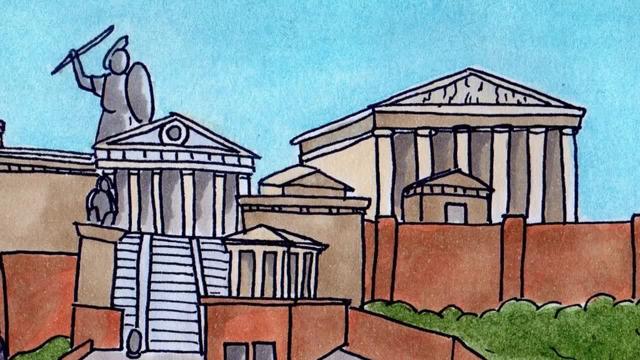 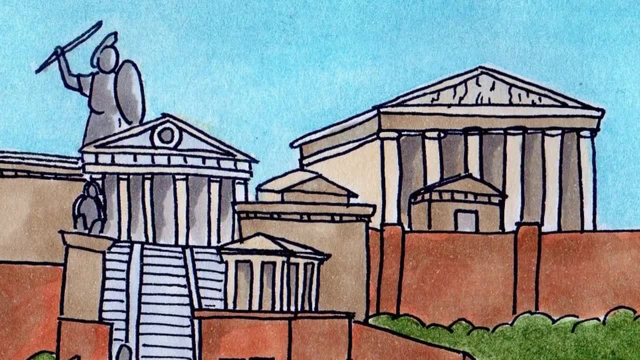 exercise and the bath-house which was next door. The Agra was ahead of her now, and then she could climb up the hill towards the temples and the Parthenon itself. Yes, Athens, It was a place where great writers could put on amazing and funny plays, or where the great sportsmen could run. 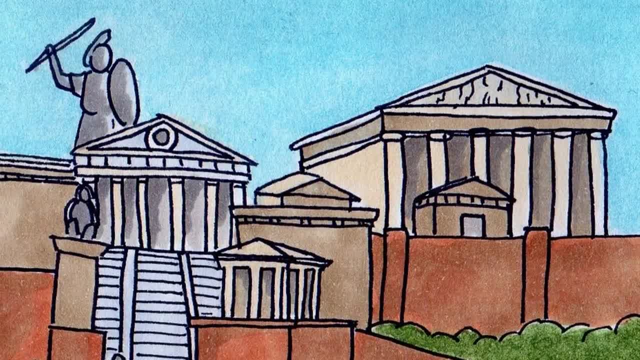 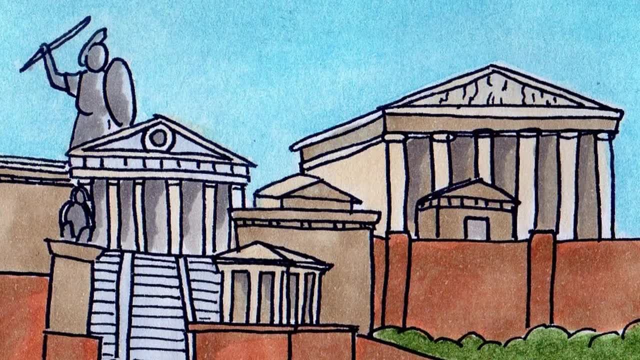 faster or throw further than anyone else in Greece. It was a place that produced the finest oils and wines in the world. It was a place where She stopped dead in her tracks. It was a place where an old man was going to be killed for. 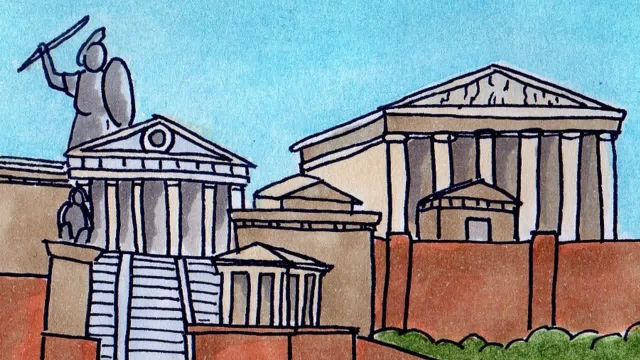 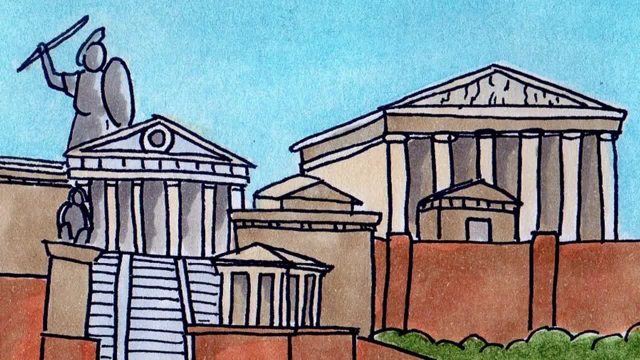 asking questions, and it wasn't a comfortable thought. It just felt wrong. Plato had been very upset and she had given him a sort of embarrassed half-hug and he had gone back to his family. She felt more confused than anything. What was it that Socrates had said, That the only 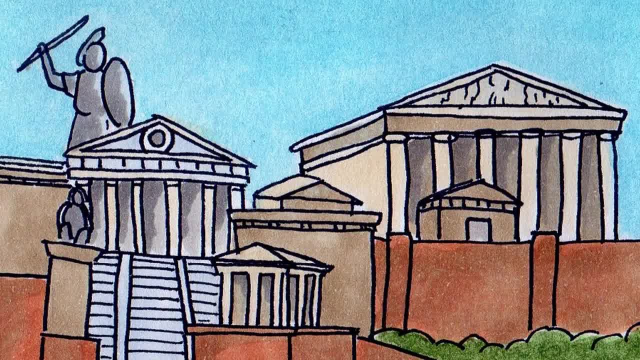 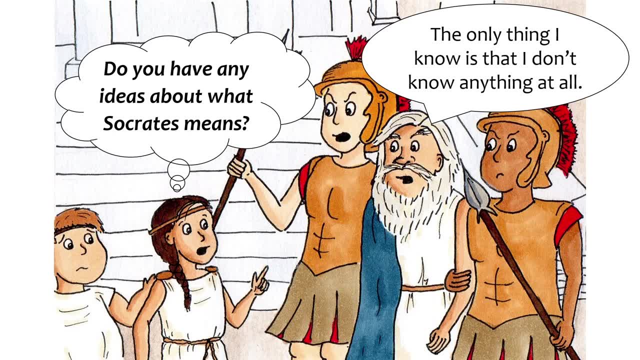 thing that he knew was that he didn't know anything at all. What was wise about thinking you don't know anything? Do you have any ideas about what Socrates means? She didn't understand, But she knew there would be someone in this city who would. It was that kind. 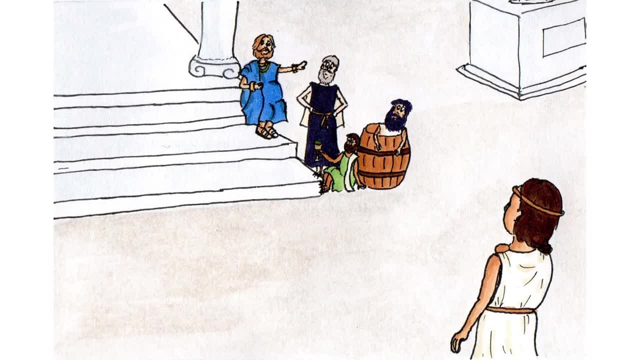 of place. That was what today's trip up to the Acropolis was all about. There must be someone around who knew Socrates, who had talked to him, who would know what he might have meant, And there was only one place that she knew of where she might find the people who she was looking for. 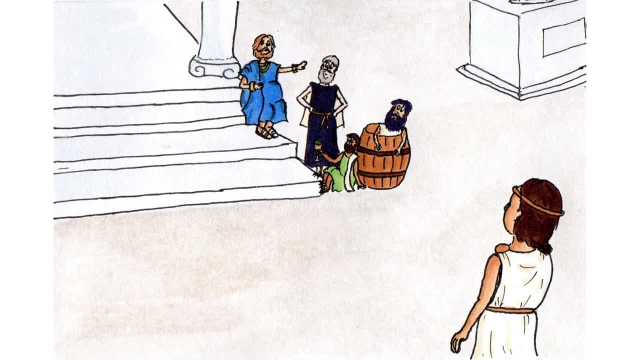 Socrates hadn't been the only thinker in Athens. after all, Socrates was the only thinker in Athens. He was the only thinker in Athens. He was the only thinker in Athens. Someone would know how to get him out of jail and back onto the streets where he. 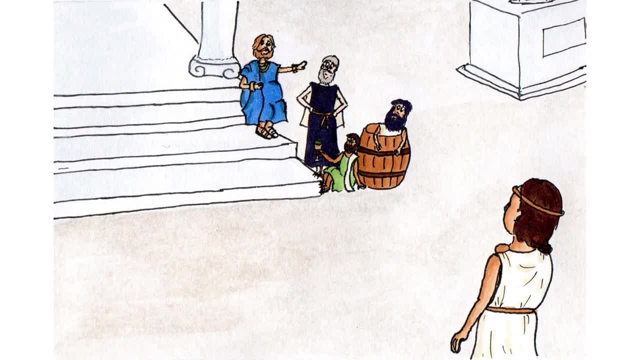 belonged. It took her quite a while to climb up towards the Acropolis. Athens stretched out below her occasional voices or clatters of stone drifting up from the rooftops. If she was honest with herself, she wasn't entirely sure who she was looking for, But she knew she'd recognise them. 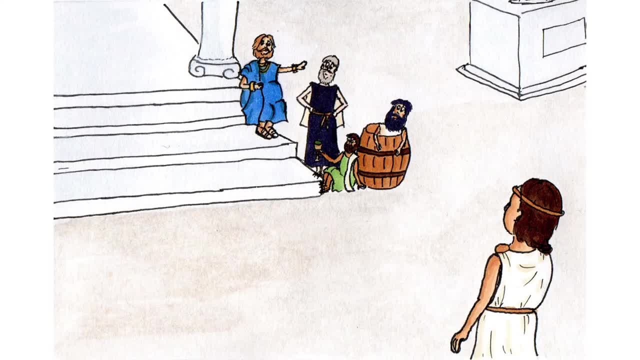 when she saw them, And she did. A small group of bearded men seated on the steps in the full glare of the sun, seemingly absorbed in a very deep conversation. They looked about right. She looked closer and doubts suddenly washed over her like a wave. In front of her were four men. 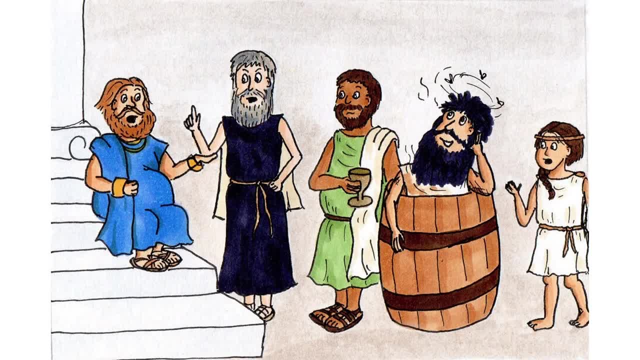 and they were some of the strangest people she had ever seen. One of them, who seemed to have a small cloud of flies buzzing round his head, was sitting inside an upturned barrel. Delphi thought he might be some sort of beggar. He was wearing little more than a filthy sheet but looked oddly cheerful. 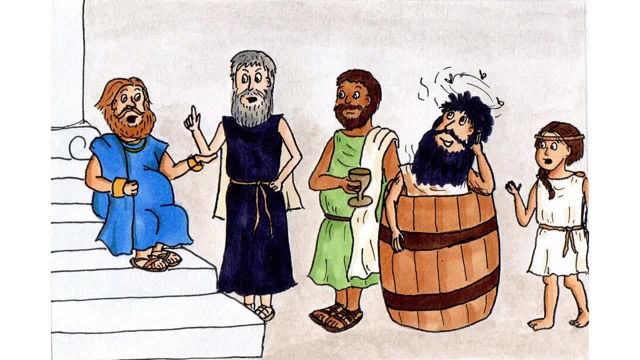 blinking into the sunlight. The second, rather cleaner-looking man was relaxing back against the side of the barrel drinking a cup of wine, looking a bit spacey. Another, a thin and tall serious-looking man dressed in black, was shouting at everyone. 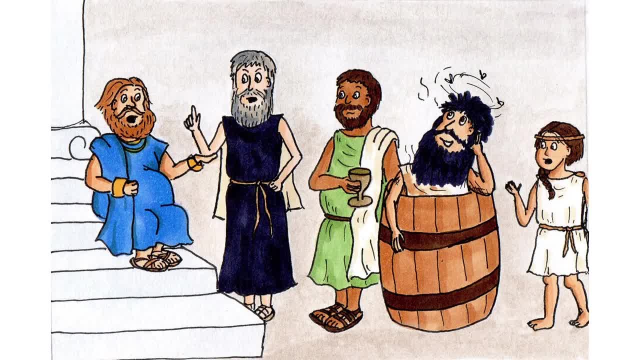 and seemed to be getting increasingly irritated that no one was listening. The last was dressed in some of the most incredibly fine and expensive clothes Delphi had ever seen. The blue-dyed coat and golden jewellery were slightly spoiled by the fact that the man was 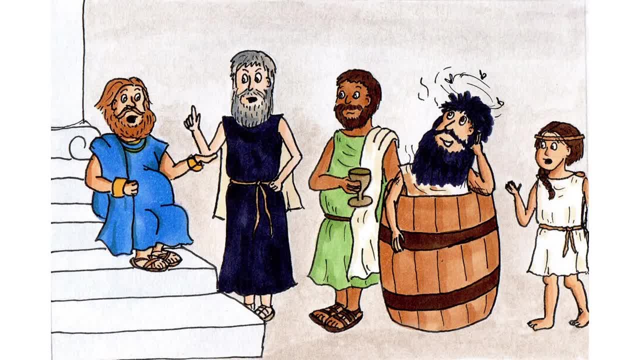 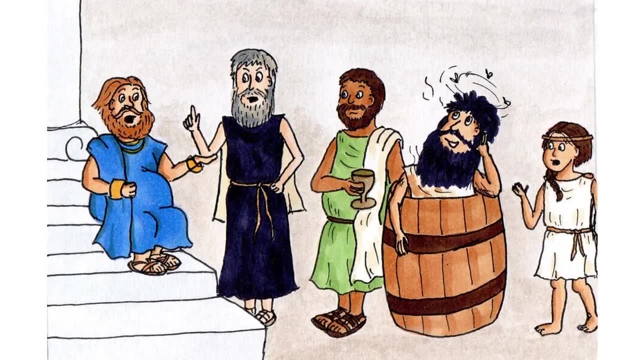 so fat that he was almost bursting out of them. All four of them had beards ranging from the tidy and trim to the wild and infested. Delphi practically froze in horror. They looked like the sort of people her dad had always told her to avoid. They didn't look angry exactly. 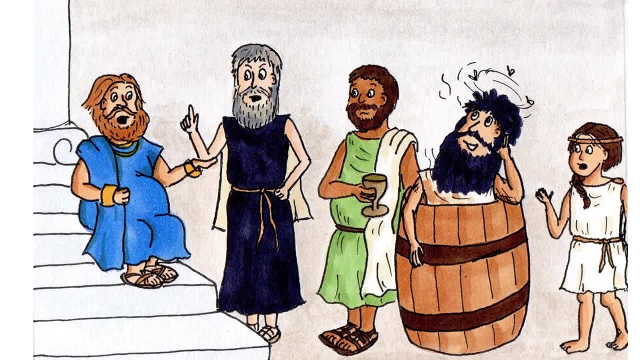 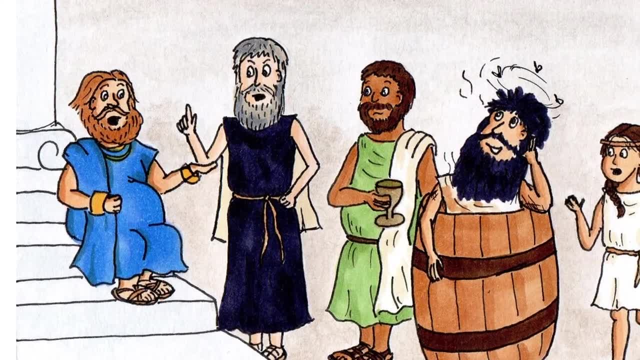 but they were all arguing about something and they were using a lot of words that Delphi didn't know. She was just about to turn and go away again extremely quickly when the fat one turned away from his argument and accidentally caught her eye. He suddenly laughed. 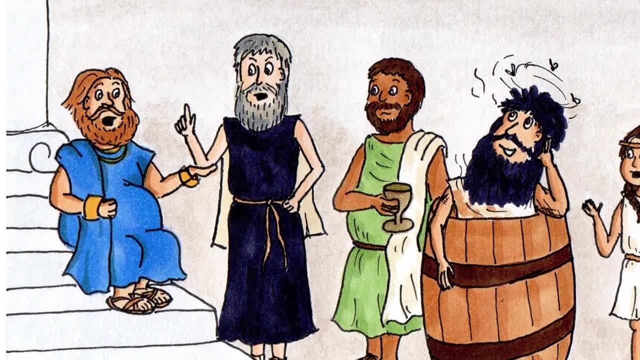 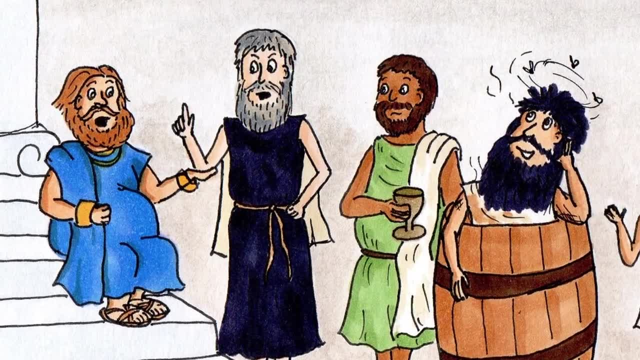 "'You child, come here' Delphi? nervously stepped forward and then stepped back again. The smell from the man in the barrel was almost overwhelming. "'Don't be afraid, my dear, I just want to ask you a question', said the fatter man. 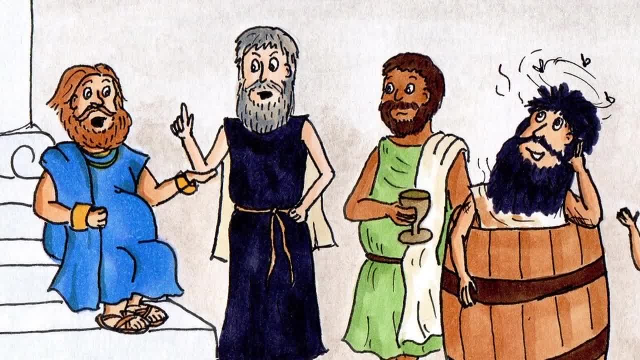 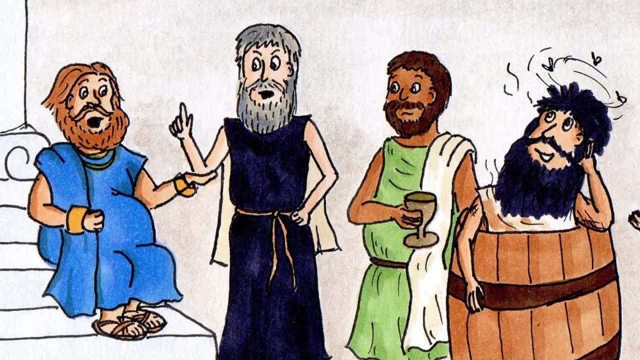 and then laughed for no obvious reason, like adults do when they think they've been good with children. "'I um actually wanted to ask you a question. I think' she stuttered and she was surprised how nervous she sounded. "'Oh really', replied the fatter man. 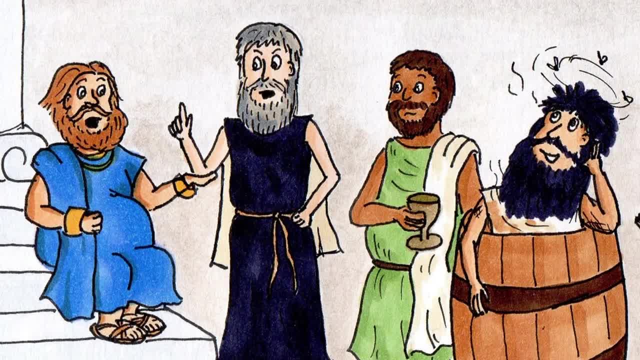 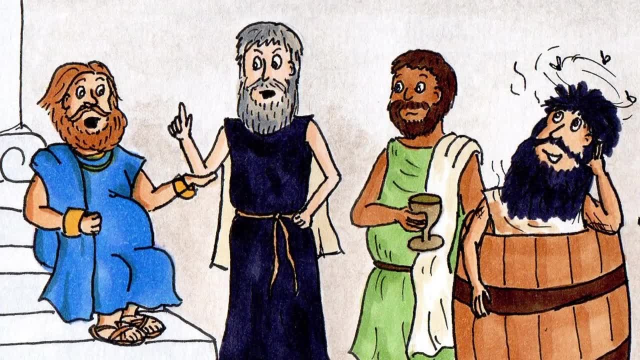 "'Well, you've come to the right place, my dear'. The man swiftly introduced himself and his friends to Delphi. She was so nervous that the names went in one ear and out the other and she immediately forgot what they were. Delphi's brain decided to start filling up the space in her mind with names. 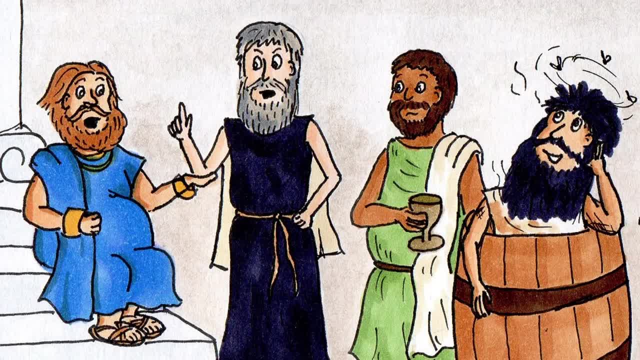 of her own. instead, Delphi desperately tried not to smile to herself as the big man in the blue robe became the fat one. "'Pah, do you really have to get children involved', the tall man said in a voice so withering it made Delphi feel about three inches tall. 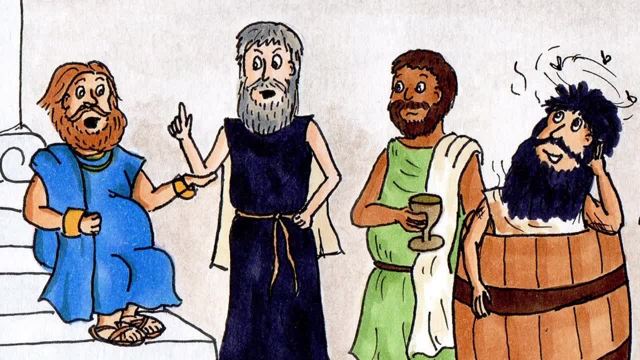 "'So he's the strict one'. Delphi thought. "'I still say that—'. The other man with the whine cut him off. "'I mean like, why not, man'. He spoke like his voice was not entirely connected to his brain. "'It's not like we can like know anything more than she can. 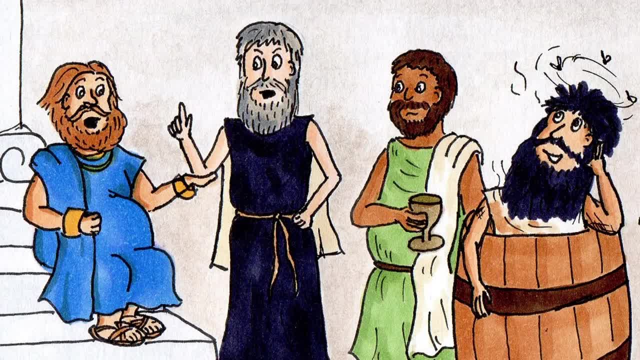 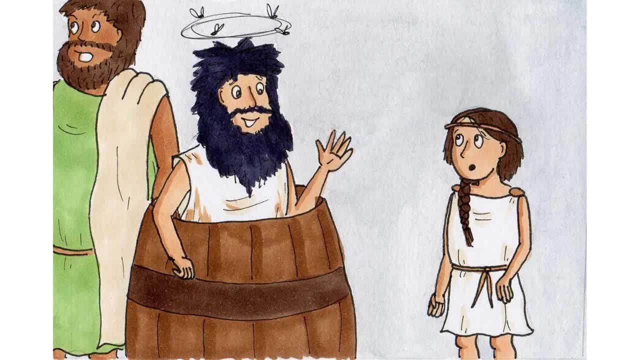 like yeah' "'The dopey one' thought Delphi. They started arguing again. Despite trying not to, Delphi found herself looking again at the man sitting in the barrel. His hair was revolting, lice seemed to be practically falling off him and he was smiling at her. 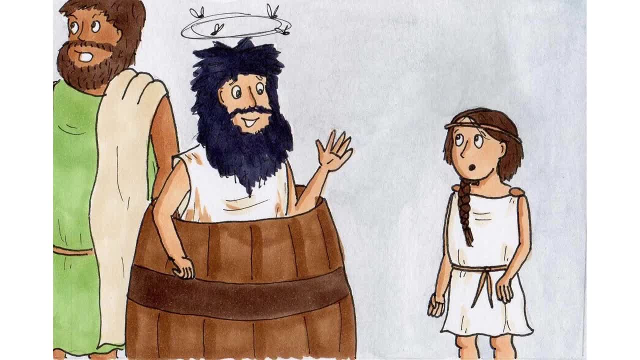 She realised she was staring and he gave a little wave. "'You're the smelly one', she thought. "'So I think I, as someone who appreciates the minds of women and children, should hear the child's question'. finished the fat one who Delphi realised had now been speaking for some time. 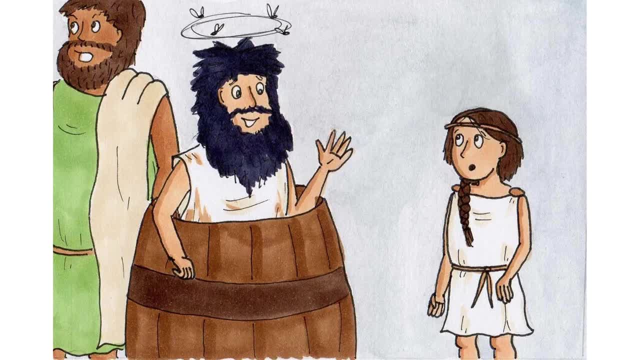 There was a brief silence. They all looked at Delphi. "'What are you exactly', she asked, still not sure she was in the right place. "'We are philosophers', declared the fat one. "'We think and we explore the biggest questions of them all. Do you know philosophy, little girl'. 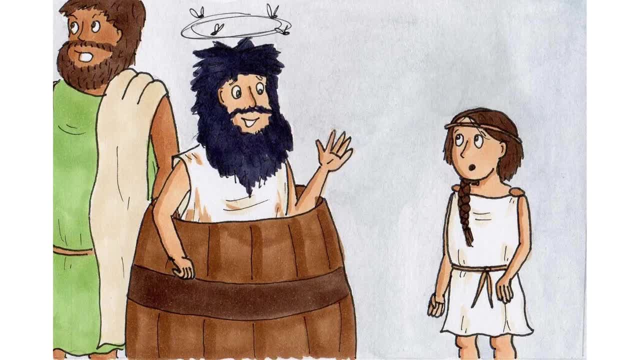 Delphi shook her head: "'What's philosophily'. "'Philosophy' corrected the strict one. "'It is the greatest thing any one can do with their mind. It is asking the most important questions in life and trying to answer them by thinking'. 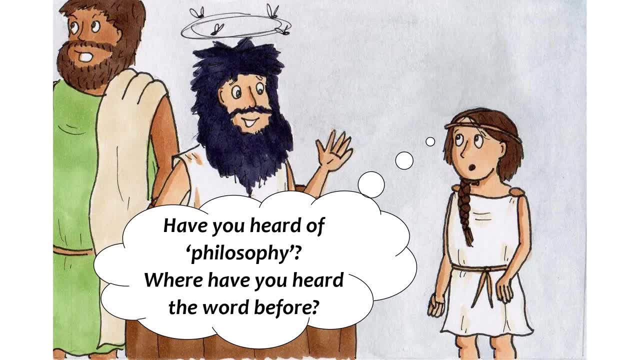 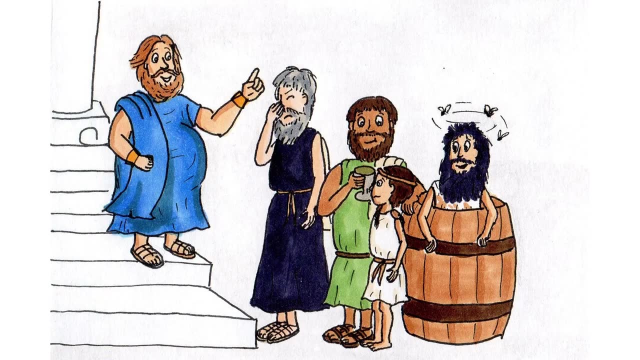 "'Have you heard of philosophy'. "'Where have you heard the word before' "'Philosophy'? "'A philosopher is someone who loves wisdom'. "'A philosopher is someone who loves wisdom'. "'A philosopher is someone who loves wisdom'. "'Wisdom, you see'. the fat one leaned down to her, smiling. 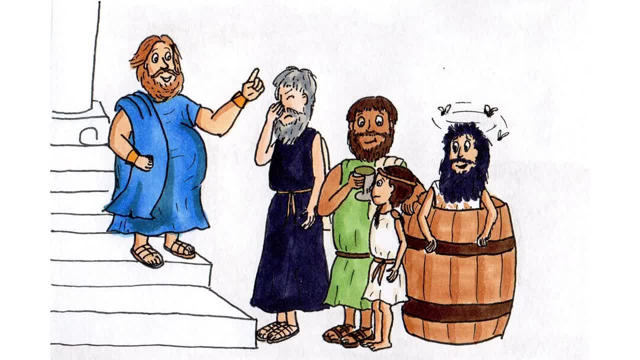 Delphi could see the sweat glistening on his forehead: "'Philo means love and Sophia means wisdom. "'Philosophia, so a lover of wisdom. you see' He laughed again for no obvious reason. Delphi could hear the strict one muttering to himself. 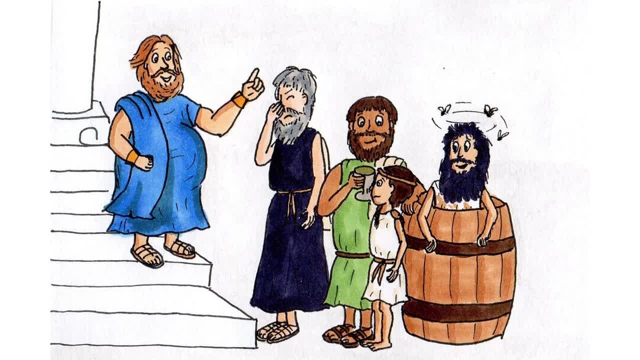 "'More like a lover of cake in your case'. "'But you can't like know for sure what philosophy is', said the dopey one. "'It's not like trying to answer everything, "'It's more like you know the questions'. 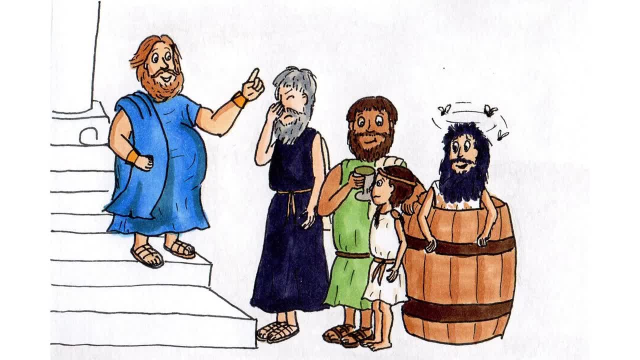 "'Questions' Delphi said, shuffling from one foot to another. "'Questions exactly', the fat one said, making his belly wobble alarmingly. "'Questions are very important to a true philosopher'. "'Yeah man', agreed the dopey one. 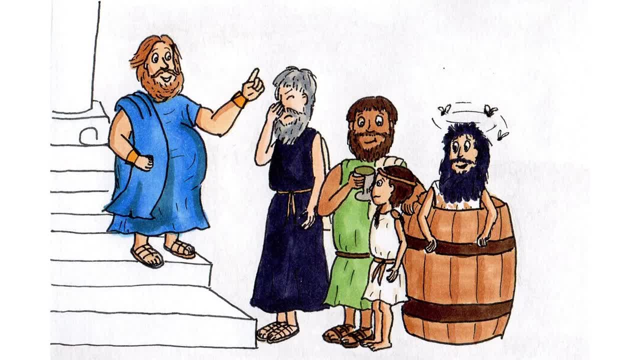 "'Like? how about this' He swiftly finished his cup of wine and invited Delphi forward. He encouraged her to sit down next to them, which Delphi did, sitting in the dirt as far away from the man in the barrel as she could. 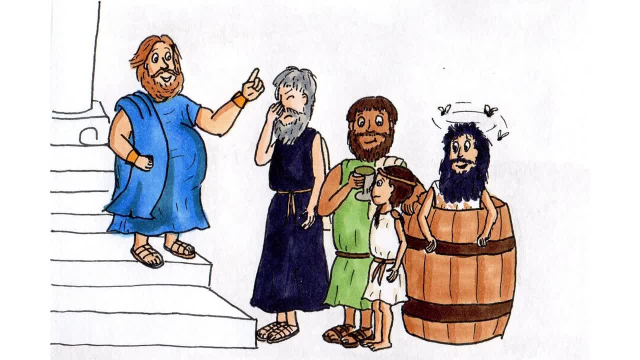 and crossed her legs rather nervously. She wasn't quite sure what she was getting into. The stones were hot on her bottom and she wondered if the stones were hot enough to hold her. She wondered if the others could smell what she could. 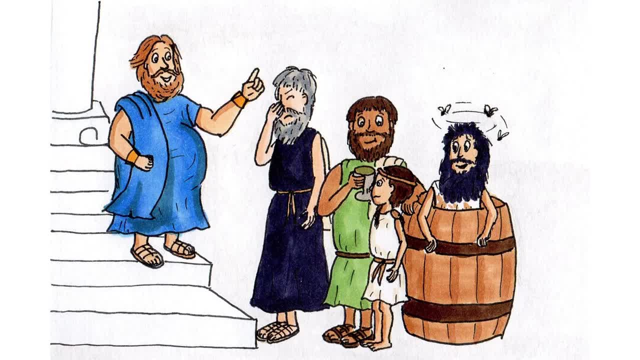 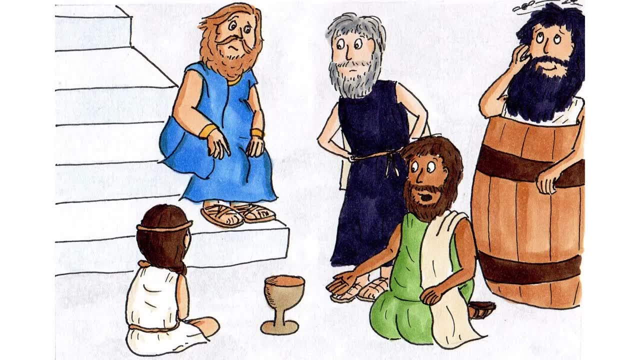 Slowly and deliberately, the dopey one put the empty cup on the ground in front of her. "'Now' he said mysteriously, sitting back down with the others. "'ask it a question'. Delphi looked around: "'Ask what a question'. 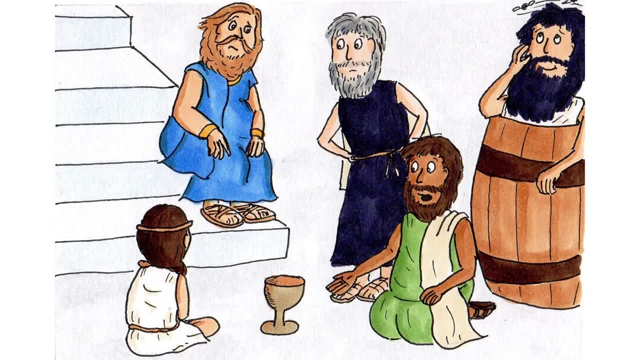 "'The cup? Ask the cup a question' Delphi blinked: "'You want me to ask questions to a cup'. Delphi wasn't sure if they were making fun of her. "'Yeah, like imagine it could answer you right. 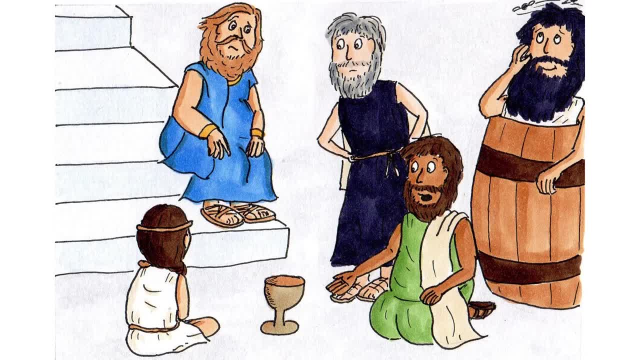 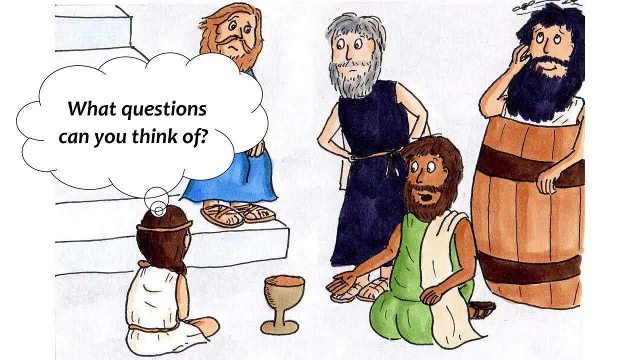 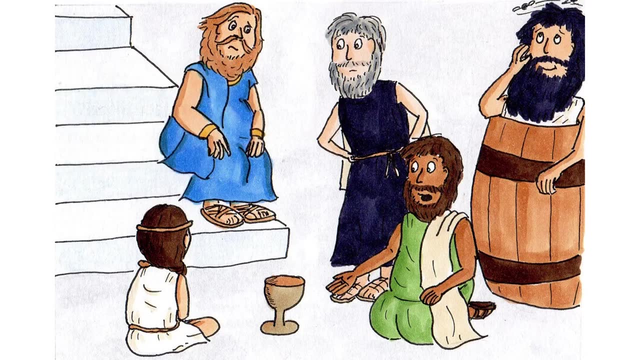 "'What questions could you ask? it that no one's ever asked a cup before'. "'What questions can you think of' "'Um' Delphi tried to think It seemed rather stupid. "'How long have you been a cup'. she tried unsure. 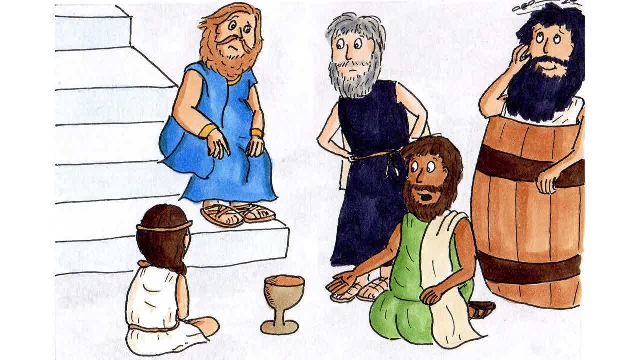 "'Good' cried the dopey one happily. "'Ask it another'. Delphi thought again: "'Do you like it'. "'Do you like being a cup' she suggested. "'Excellent, Be more precise, if you can' chipped in the fat one. 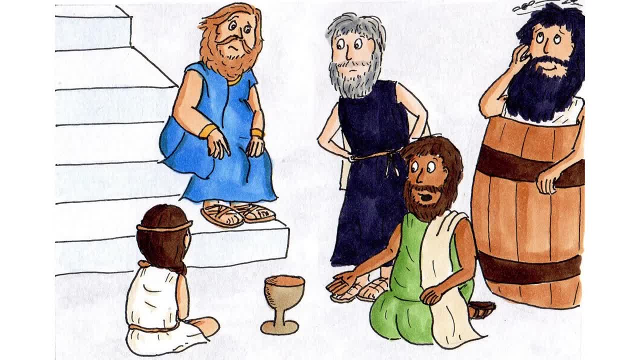 "'Um, what's it like when someone drinks out of you'. She paused, looking at the philosophers. "'Well, keep going if you're going to', snapped the strict one, looking rather impatient. "'Oh, um'. Delphi tried to think faster. 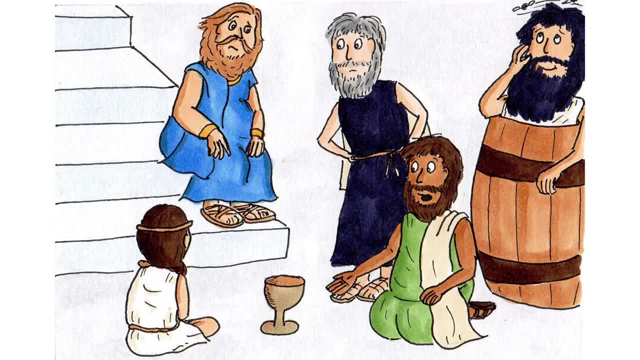 "'Do you prefer holding water or wine inside you? "'Uh, would you like to be bigger? "'If you couldn't be a cup, what would you rather be'. She paused for breath and the men seemed to be nodding. "'Are you one thing or lots of things' 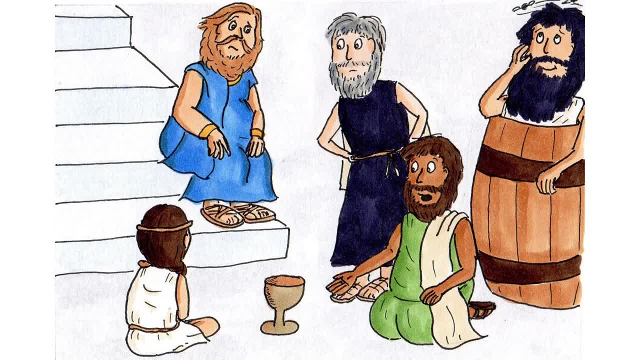 suggested the fat one. "'Would you be the same thing if we called you a hat', asked the strict one. "'Are you really there or does it just like? look that way' drawled the dopey one. Delphi looked at the man in the barrel, but he appeared to be dozing in the sunshine and 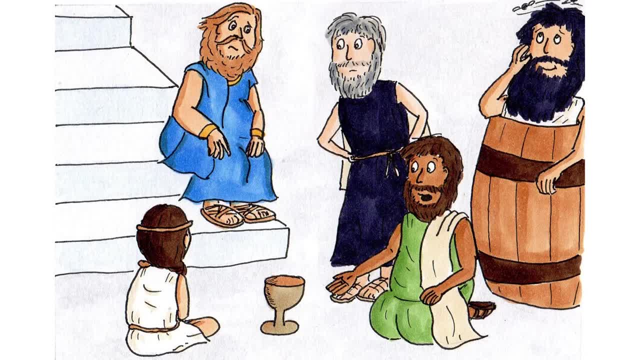 wasn't listening. "'You see' said the dopey one looking pleased with himself. "'There, we have, just like, asked some of the biggest questions there are'. "'I don't understand', admitted Delphi. "'Of course you don't. 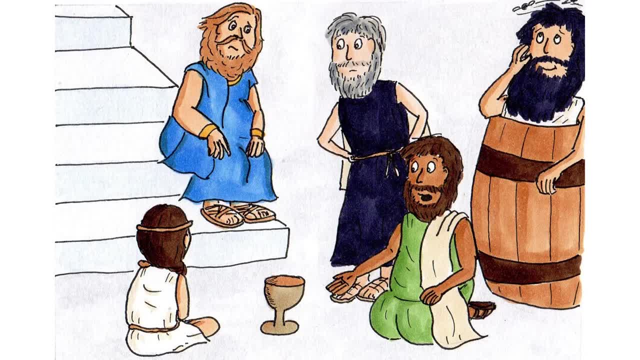 You're just a child' said the strict one, sneering a little. Delphi shot him an annoyed glance. They didn't seem to notice. "'We call them philosophical questions', said the fat one smiling at her. "'Questions don't have a simple answer, but we can get better answers by thinking about them'. 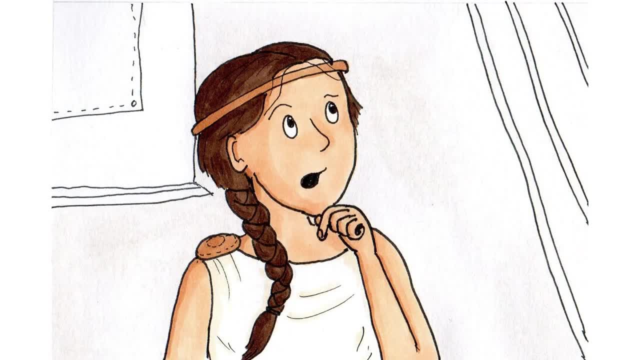 "'Philo—physilo—phi—' tried Delphi. "'Big questions—' cut in the strict one. "'Just call them big questions' "'Big questions, right', agreed Delphi. "'So questions don't have a simple answer like: why is my dad always grumpy'. 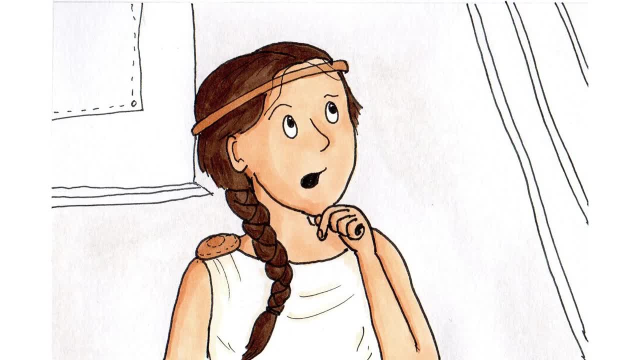 the fat one seemed to think for a minute: "'Possibly, Possibly Stick with. why That's a good start' "'Why' Delphi looked around, Athens gleamed. "'Why are there so many people? Why aren't women and children allowed to go out during the day'? 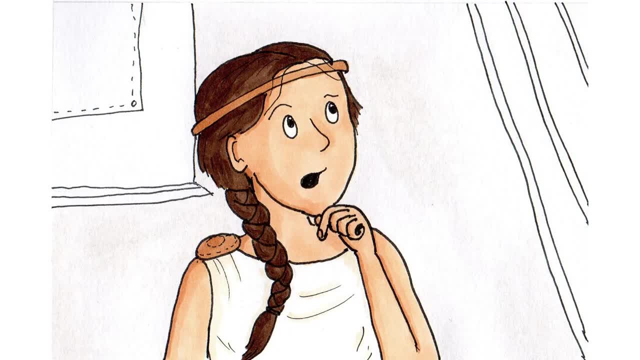 "'Yeah' laughed the dopey one. "'Bigger Sillier'. Delphi's mind started to race. "'Why is the sun so hot? Why do we have to pay for things? Why can't I eat all the honey cakes in the world'. 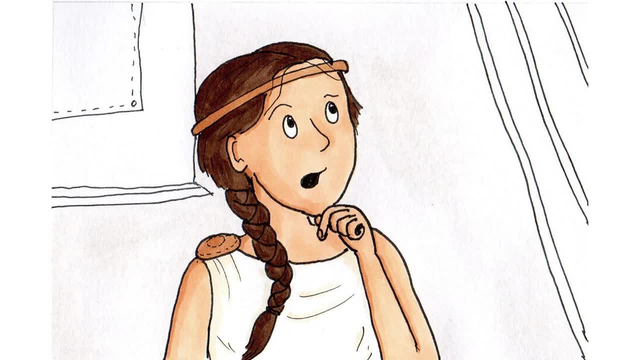 she giggled and was surprised to see the philosophers laughing along with her. "'Good, Keep going. You're getting it', cried the fat one. "'Not just why? How? What if'? Delphi could feel her heart beating and, slightly to her surprise, she realised she. 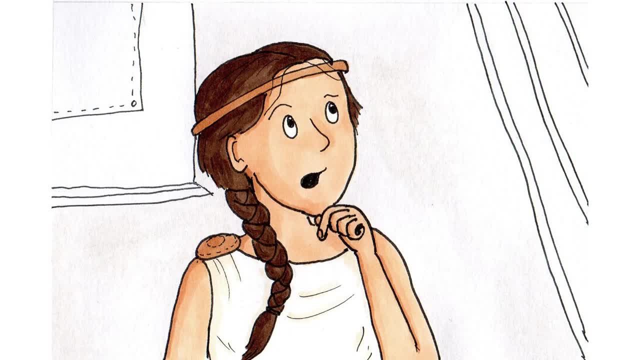 was enjoying herself. "'How can you talk to the birds? What if I was a princess? Would I be different if I was a dog'. Delphi gabbled, speeding up. "'Um, Why can't I live forever'. "'You see, the girl's a natural philosopher', declared the fat one, beaming at his companions. 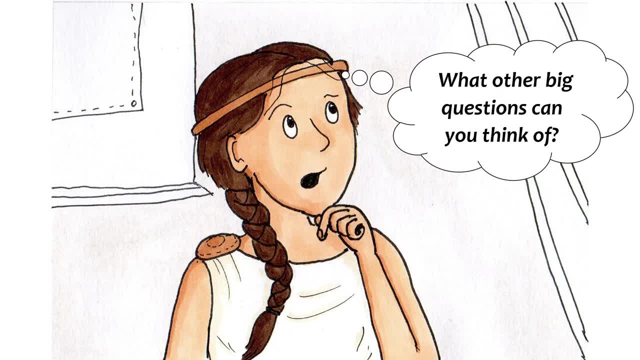 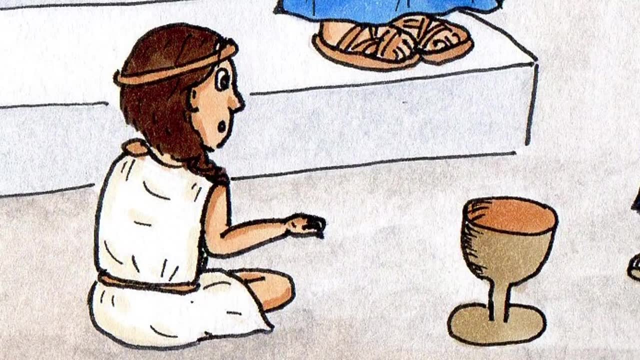 "'Keep going'. "'What are the big questions can you think of'. Delphi's questions seemed to be coming quickly now. It was funny that once she got the hang of it, it really wasn't very difficult. She was almost out of breath. 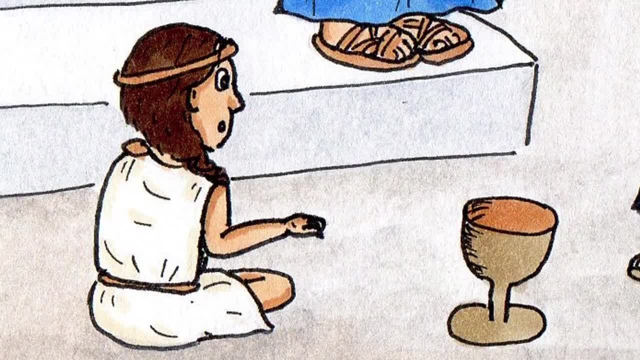 "'Why are things different colours? Why isn't everything the same colour? Why is red more red than blue? What does red taste like? What does blue taste like? What does green taste like? What does yellow—'? "'Yes, yes. 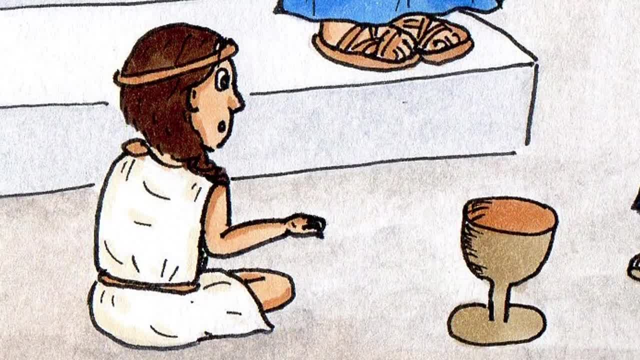 Well done' interrupted the strict one, wiping the sweat off his forehead. "'You seem to have got the idea'. Delphi stopped talking and realised they were all staring at her. She took a few deep breaths. "'So that's—'. 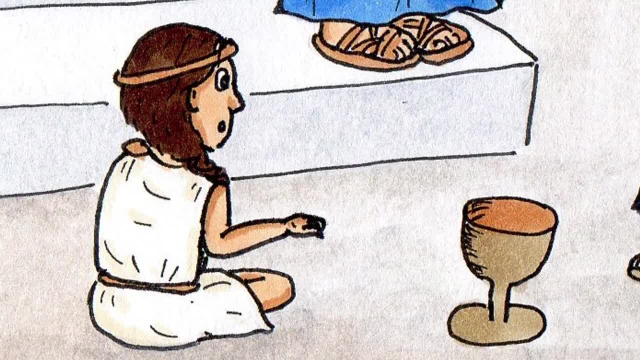 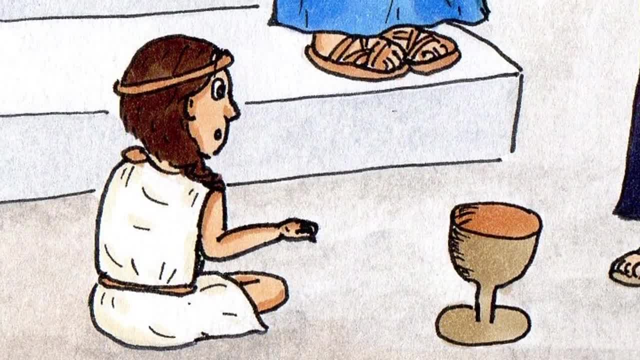 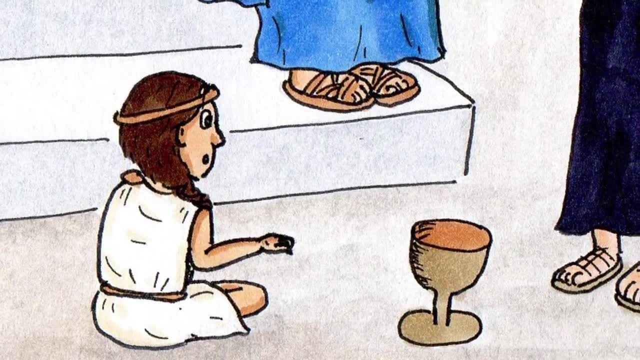 fat one leaning back on the steps. "'Just asking cups how they feel and how big the sun is, and stuff'. "'Ah', the strict one held up a finger. "'Be careful, The size of the sun is not really a philosophical question. 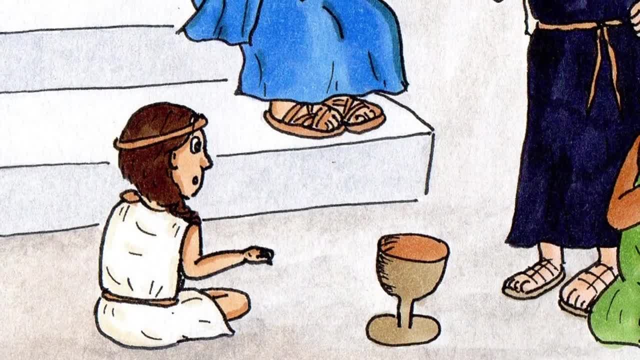 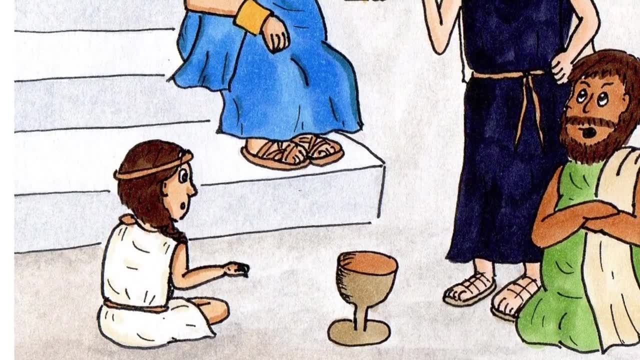 We can't learn more about it by thinking about it? you see, We would need a—' he waved his hands around—'an extremely large ruler to find out how big it is, but it would have one definite answer: Perhaps one day we'll know. but there isn't much to discuss until somehow we can go and 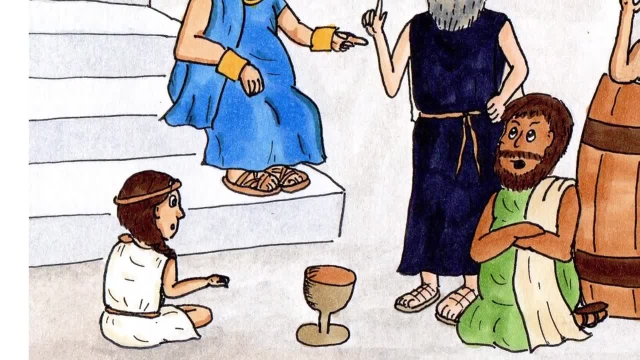 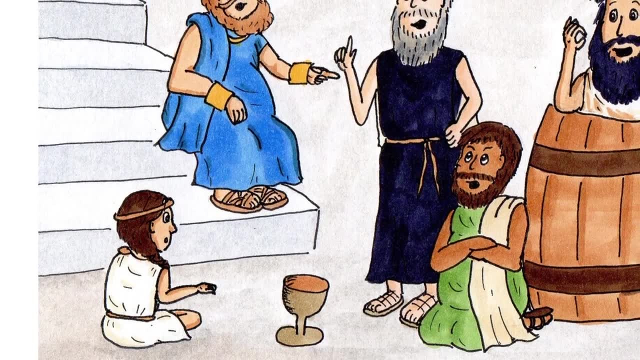 measure it, whatever it is'. "'Oh right'? Delphi nodded. "'That seemed to make sense, except the bit about the giant ruler'. "'Now what was it we were going to ask you', said the fat one. There was a groan from the strict one. 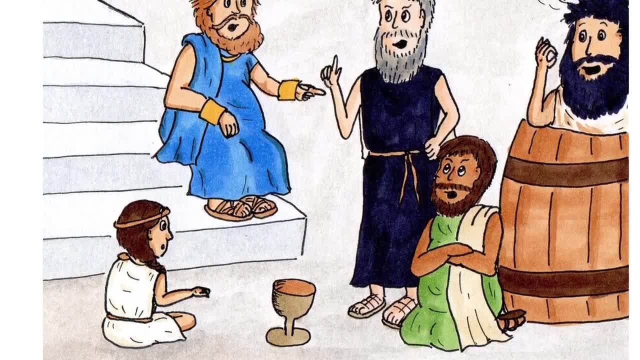 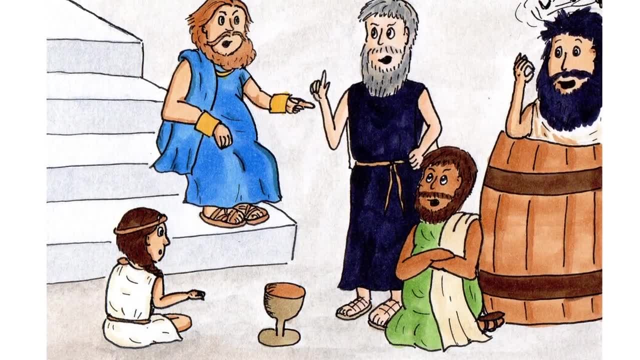 "'Oh yes, What would you say is the best way to live? How do you become a good person'. They all looked at her. Delphi blinked: "'That's weird. I was going to ask you that. You see, I met Socrates. 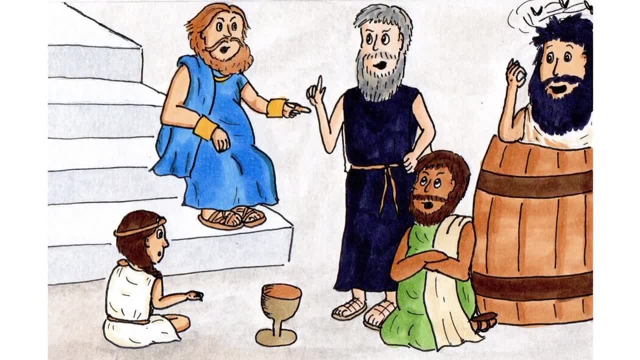 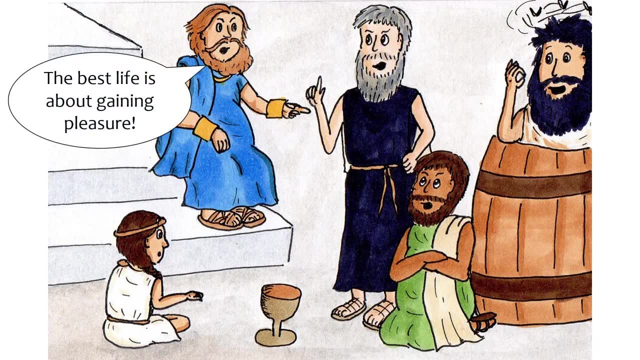 He said: "'Ah, Socrates' sighed the fat one. Now there's a man who could ask a good question. So what do you think'. Delphi thought for a few seconds "'I—'. "'I say the best kind of life is the one where you gain as much pleasure as possible'. 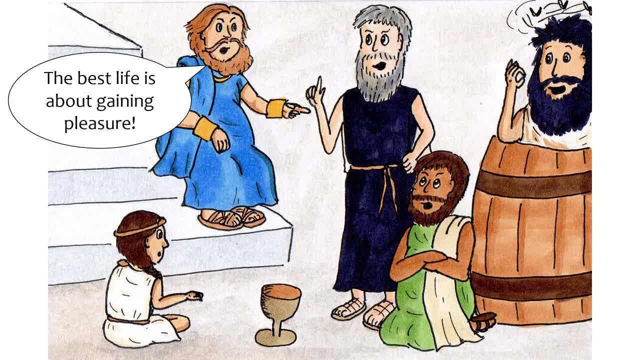 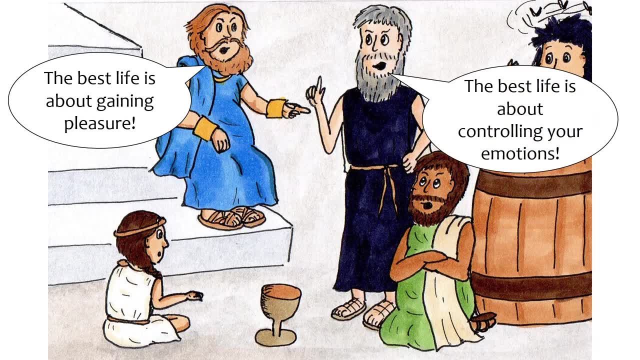 the fat one boomed while Delphi glared at him. "'Nonsense', declared the strict one standing up. "'I say, the best life is where you control your emotions and desires and live as sensibly and as rationally as possible'. 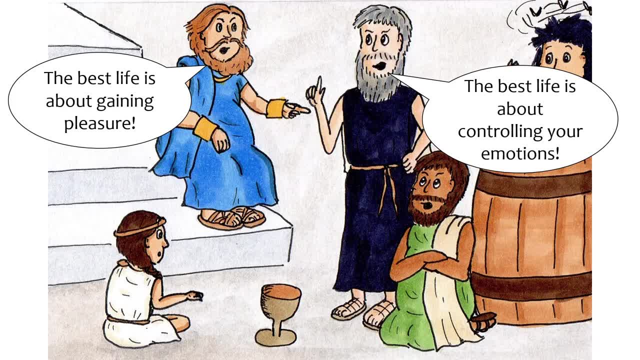 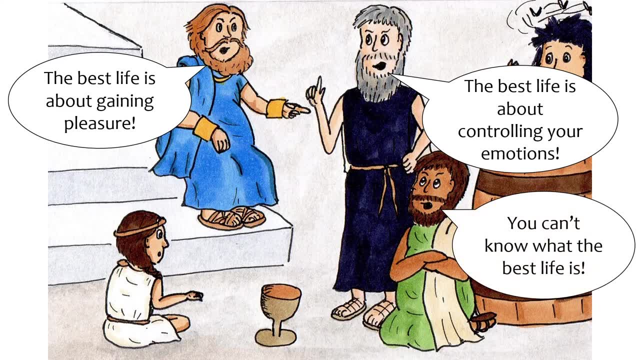 "'No, no, no' the dopey one had stood up and was waving his hands around, "'You can't like know the best way to—'. "'You can't like know anything'. The smelly one was watching them all happily, but didn't say anything. 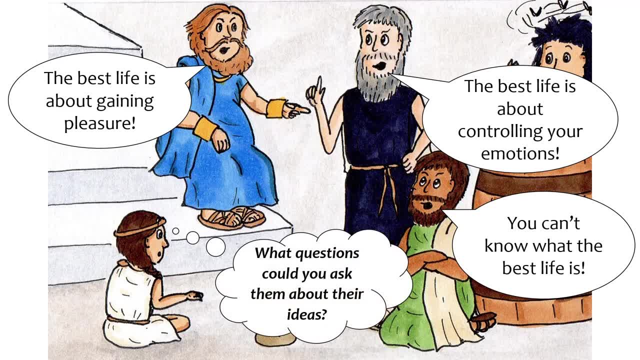 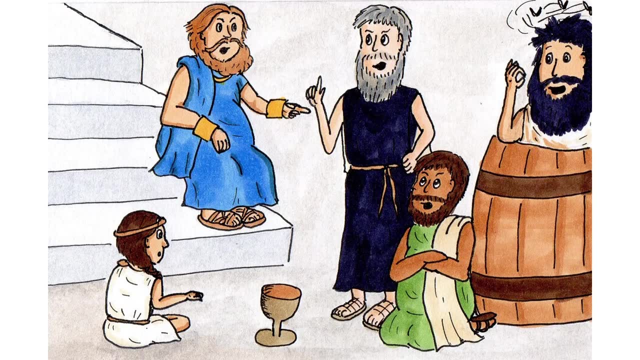 "'What questions could you ask them about their ideas'. "'So you don't know', Delphi asked. "'All three of the philosophers slumped a little. "'It's not that we don't know exactly', muttered the fat one. "'It's more that we don't agree' said the strict one. 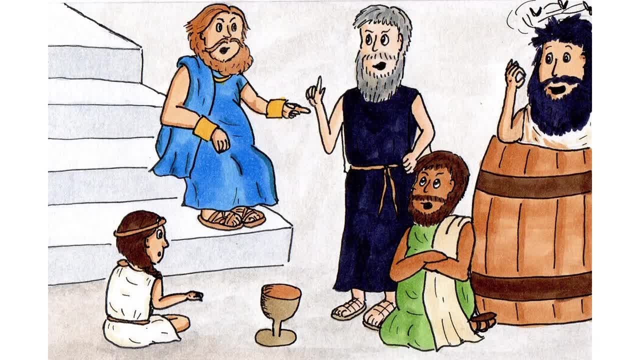 "'But that doesn't matter. That's just what being a philosopher is all about'. the fat one said, smiling: "'Nothing wrong with not agreeing with each other. Ideas get better if you have a good argue about them. It's not an unkind thing to do, as long as you do it right'. 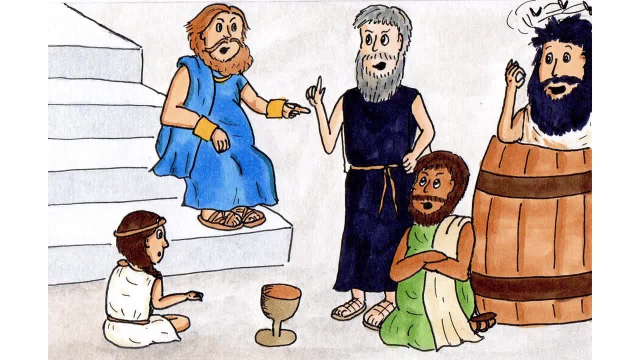 "'It is true, that is why you find us here today'. the strict one said. "'Just like, exercising strengthens the body, talking about ideas strengthens the mind, Socrates—'. Delphi understood that much at least. "'He told me that the only thing he knows is that he doesn't know anything', said Delphi. 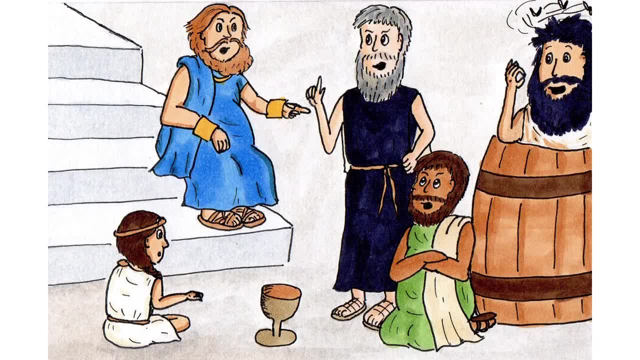 "'What did he mean by that'. All three of the philosophers took a breath and started talking at once. "'Well, I think that that's clearly wrong, because obviously he meant that—'. "'Oh, forget it', Delphi snapped. 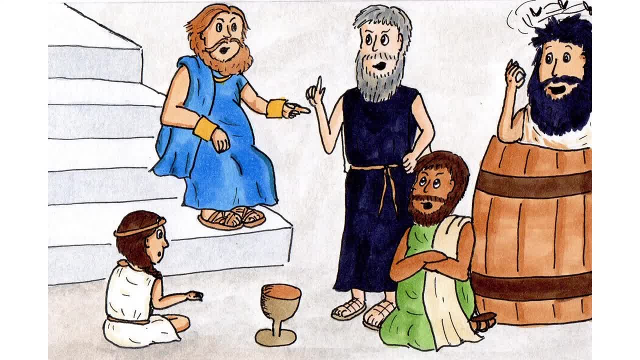 She hadn't heard a word of what they said and she doubted whether it would have been useful. anyway, Maybe they could answer one question at least: "'Why are they going to kill him' Delphi asked. There was a brief, uncomfortable silence. 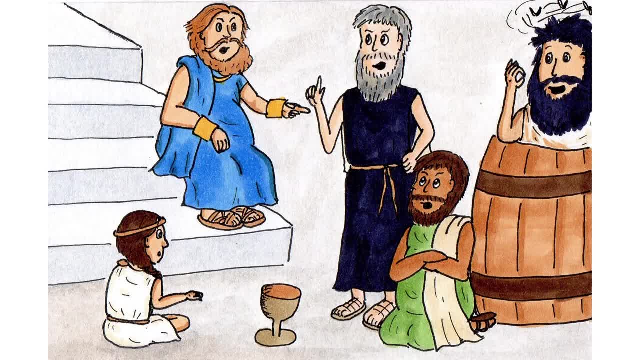 Delphi wondered if she had said the right thing. "'It was that Miletus', the fat one suddenly roared the layers of his middle, wobbling like an earthquake as he tried to stand up. "'That jumped-up beaked-nosed little—'. 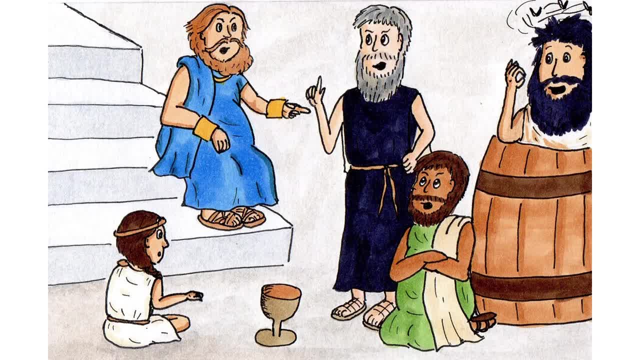 "'Quiet', hissed the strict one at him. his teeth clenched. The fat one shut his mouth after a couple of attempts. The dopey one was just staring at the sky. "'Some questions', the strict one started looking at Delphi. 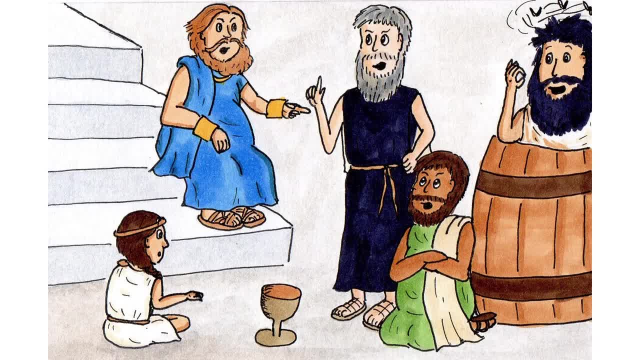 "'Are not good to ask No more questions from little girls today, I think'. Delphi blinked. "'Why not'? "'Enough', the strict one suddenly looked furious and leapt to his feet. "'Why not', he said. "'Leave us be. You are lucky. we have given you as much time as we have'. 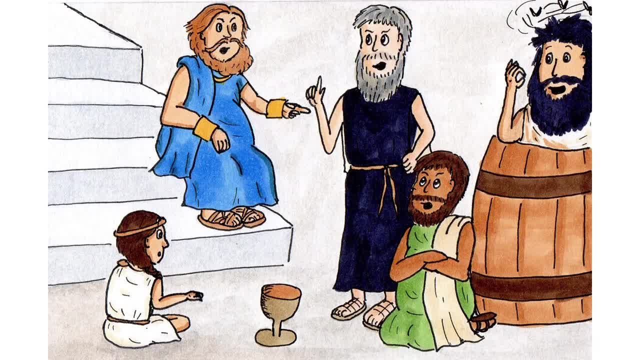 "'Yeah, controlling your emotions, right', said the dopey one smiling. The strict one stopped open-mouthed. "'Better go, kid'. the fat one suggested finally on his feet. "'Thanks for your questions, but take them somewhere else'. 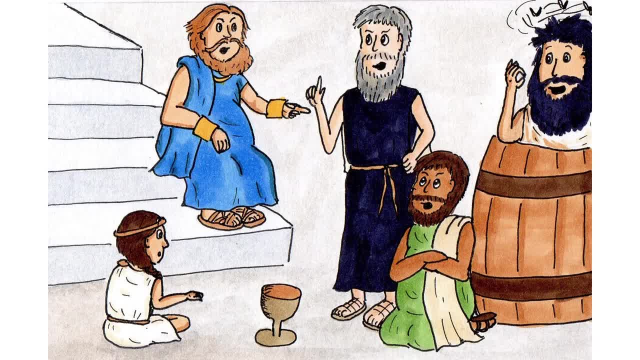 "'But I need to know—'. Delphi felt the anger burning up inside of her. It was a fire that had been burning hotter ever since Socrates' trial. "'I need to know what he was looking for. I need to know because I'm going to be a philosopher like him. 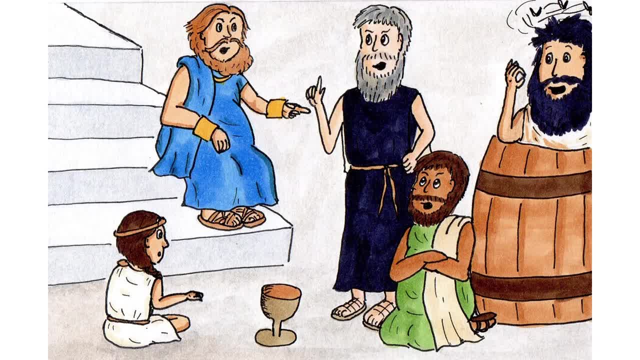 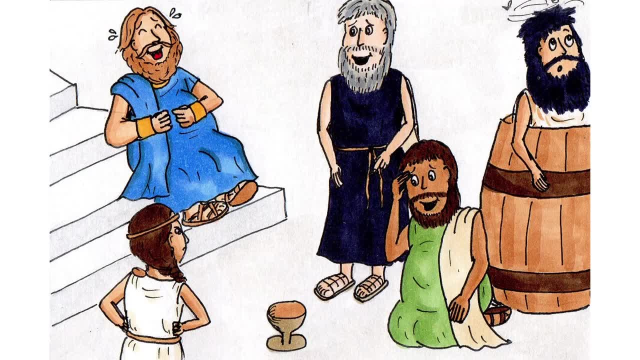 and I'm going to get him out'. To her horror, the three men suddenly burst out laughing: "'You' the strict one, sneered, "'You're just a little girl. I bet you can't even read'. Delphi was squeezing her fist together so hard that she felt her fingernails pinch into the. 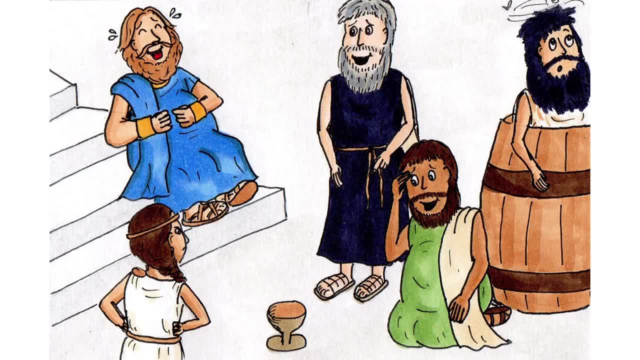 palm of her hand. "'Yes' she shouted. "'Some one has to, and it looks like no one else in this stupid city is going to do it'. The fat one was wiping some tears out of his eyes from laughing so hard. "'Go on, little girl', he said, sitting back down again. 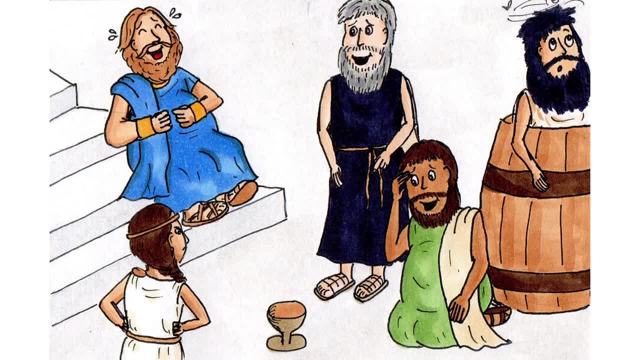 "'Do come back and tell us when you've persuaded the entire city to let him go'. Delphi took a few deep breaths. She was astonished how angry she felt. If someone had called her a philosopher this morning, she wouldn't have known what they meant. 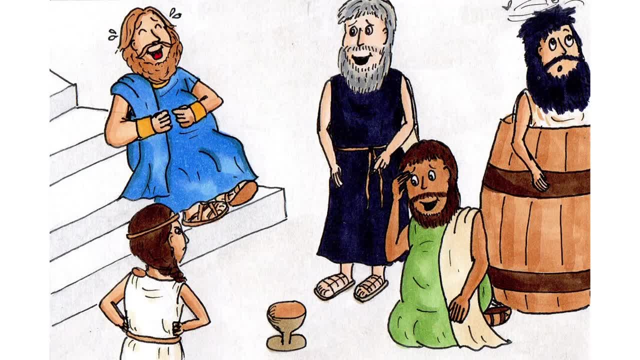 Now, the thought of not being one was unthinkable. She turned to go, the laughter echoing in her ears. She managed a few steps back down towards the streets before a thought hit her. She stopped. She turned around again and marched back up to the smelly philosopher in the barrel. 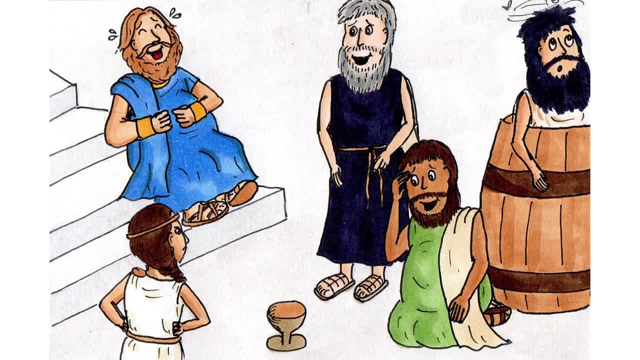 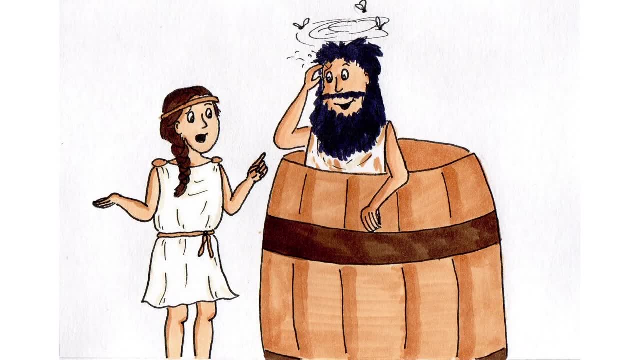 who was still smiling in the sunlight and hadn't said a word the entire time she had been there. She stood in front of him, hands on her hips, casting a shadow over him. "'What do you think', she asked. "'Are you even okay? Do you need anything' 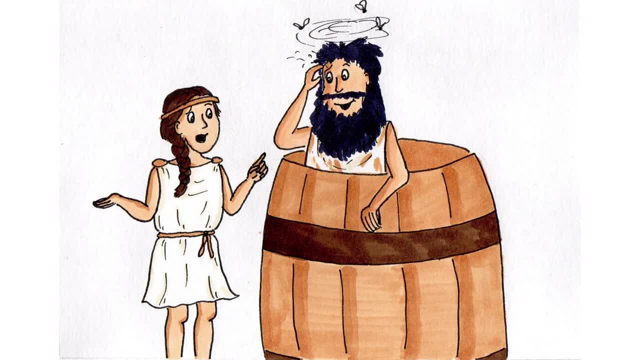 The man scratched his head, sending little white flakes down to his muddy knees. "'Please' he said his voice gravelly but clear. "'Please' "'Yes'. Delphi leaned closer. She held her breath to try and stop the smell getting in, but it did. 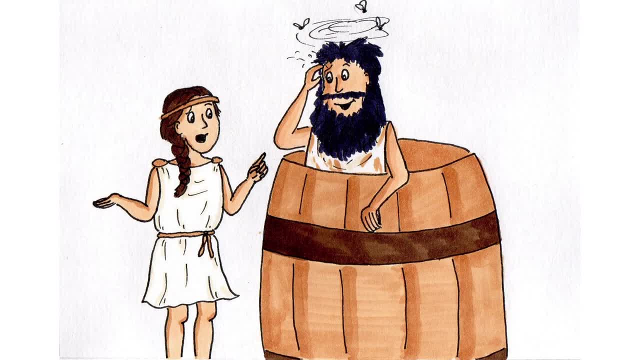 "'Please'. "'Stand out of my light'. Delphi felt confused for a moment, then realised what he meant. "'Oh sorry', she said, stepping aside allowing the sunlight to warm her face. Delphi would never know this, but funnily enough. 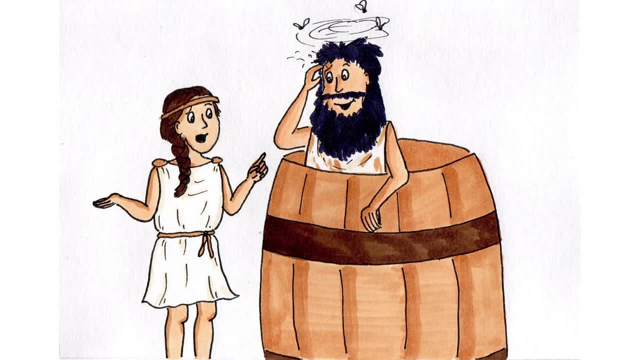 he would give exactly the same answer to Alexander the Great. when asked the same question. His real name was Diogenes. He smiled and looked as happy as any person she had ever seen in her life. "'Could you be happy if you live like Diogenes?